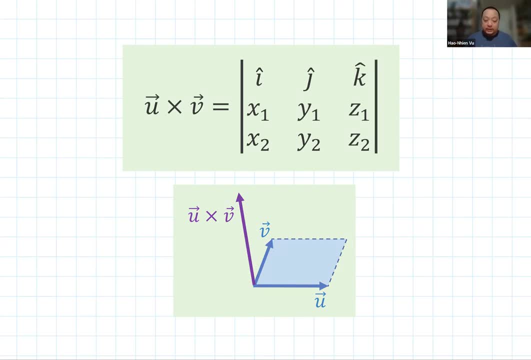 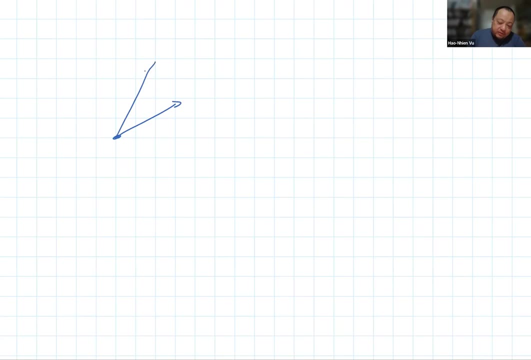 my other videos. so I'd like to thank my viewer for that. Okay, so I have two vectors- u, v, in space somewhere. They're in space somewhere flying around, and now I'm going to take u cos v. I will end up with a vector w. That vector is perpendicular to u, perpendicular to v. 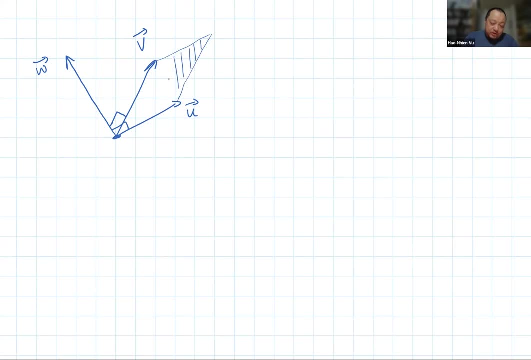 and supposedly has a length that's equal to this area. Remember that the cost product is defined as the determinant i, j, k, x1, y1, z1, x2,, y2, z2, where the x, y, z are the coordinates. 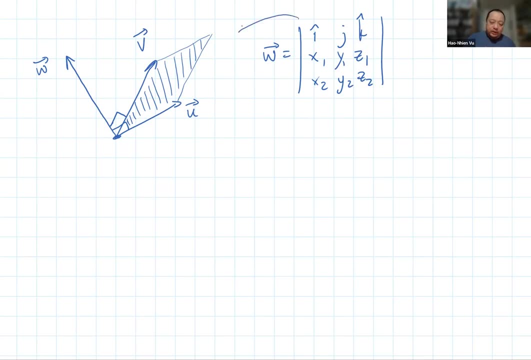 of the vectors. So I'm going to have to prove that this determinant is equal to that area. Well, you have the u and v flying around in space like that. Who knows where the x, y, z axes are? So I might have. 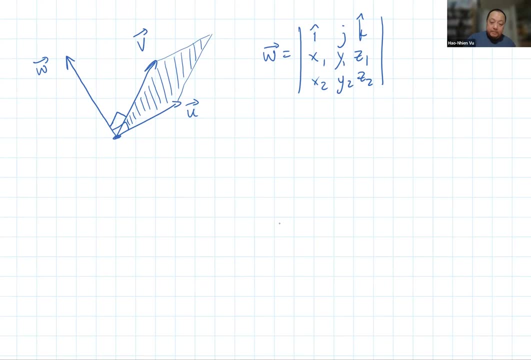 to define it in a way that's easy for me. I'm going to define the origin as this point, right here. I'm going to define the x-axis as the axis that goes along the direction of the u vector. I'm going to define the x- y plane as the same as this plane, And so the y-axis will be on that plane. 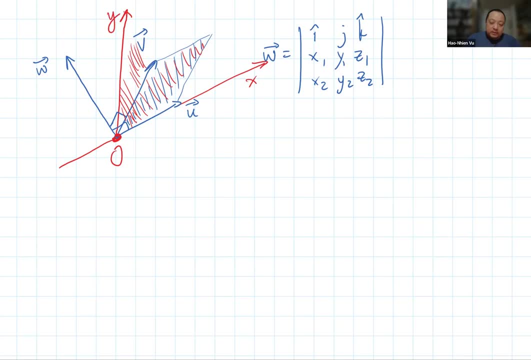 somewhere is on the same plane as both the u vector and the v vector. Once I have defined my axis, that way I can redraw the picture in the new x- y plane. Here's my x-axis. Here's my y-axis. My vector u is going to be here because that's how I defined. 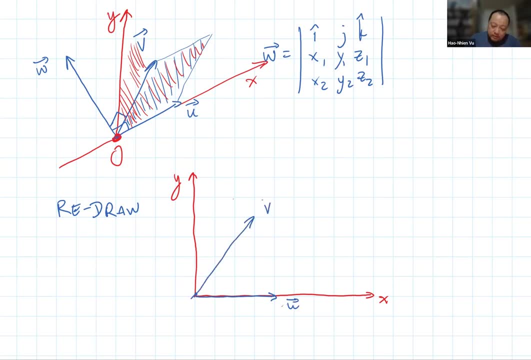 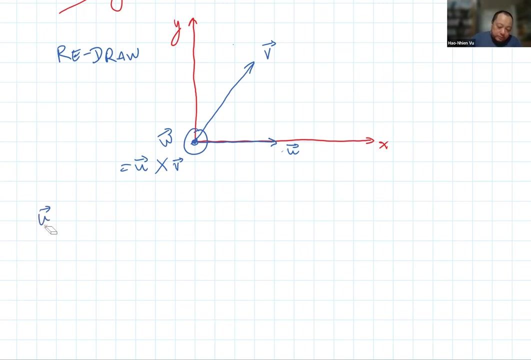 the x-axis, v is somewhere on the same plane, because that's how I defined it, And w will be sticking out of the page looking at us And w is u cross v. Given those axes x and y, then u is equal to sum x1, 0, 0.. x1 is this position here. 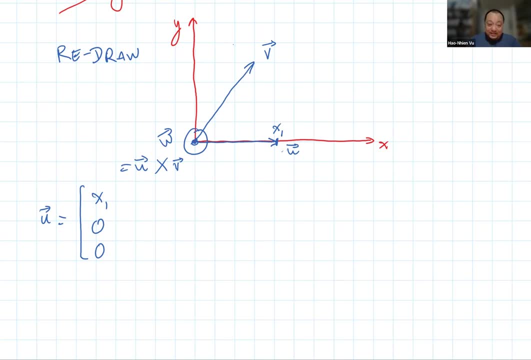 And because it's on the x-axis, then the y coordinate and the y and the z coordinates are 0.. The vector v is on the x- y plane, so it has some sort of x coordinate, some kind of y coordinate and 0 on the z coordinate. So here's x2.. And here's y2.. Then u cross, v will be the. 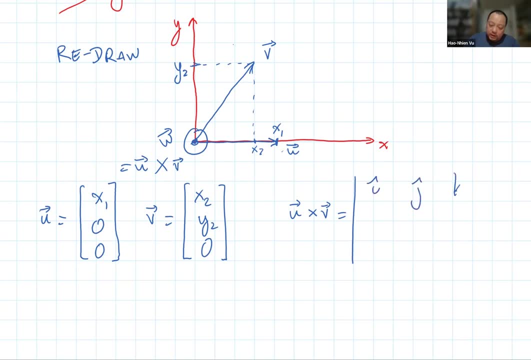 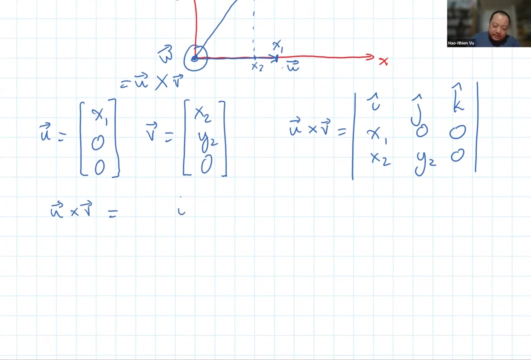 determinant i, j, k, x1, 0, 0, x2, y2, 0.. I work this out. I get u. cross v is equal to. First of all, I need something on the i. 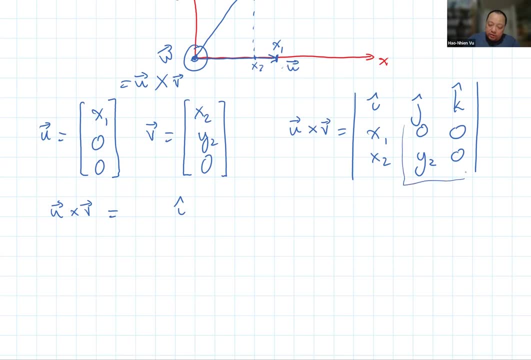 coordinate. Well, on the i coordinate, is this determinant, And that's just 0 minus 0.. So the whole thing is 0.. Minus something on the j coordinate. On the j coordinate, I have this product and that product, And that's also 0. 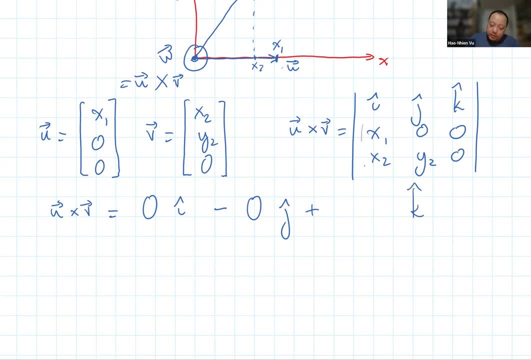 On the k coordinate I have this determinant: x1, 0, x2, y2. And that is equal to x1, y2 times k. That's the cross product of u cross v, So the length of the cross product. 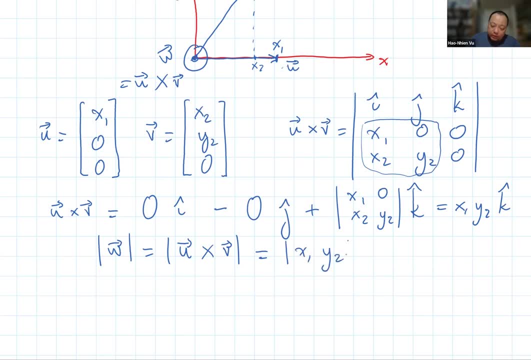 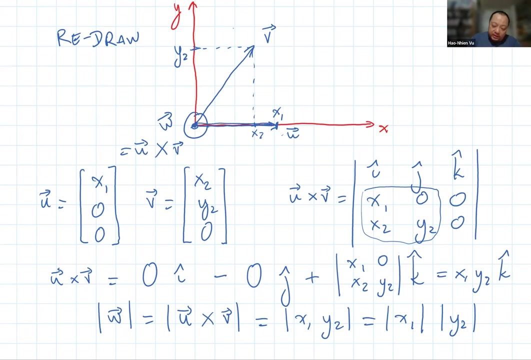 is the absolute value of x1 times y2, which is the absolute value of x1 times the absolute value of y2.. Let's now take a look back at this picture and see what x1 is. x1 is this length, right here? 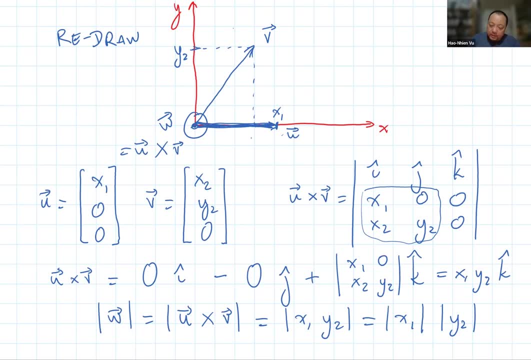 x2 is no longer in the picture, so let me erase that. And y2 is this length here, which is also this length there. And if I draw the parallelogram, then x1 is the base and y2 is the height of the parallelogram. 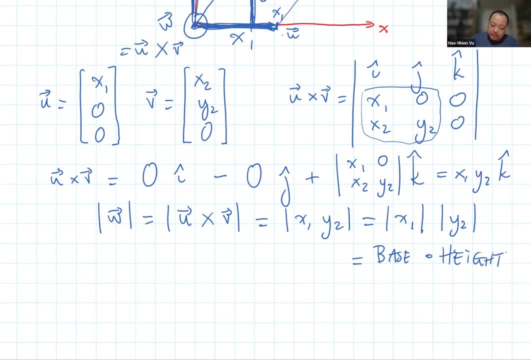 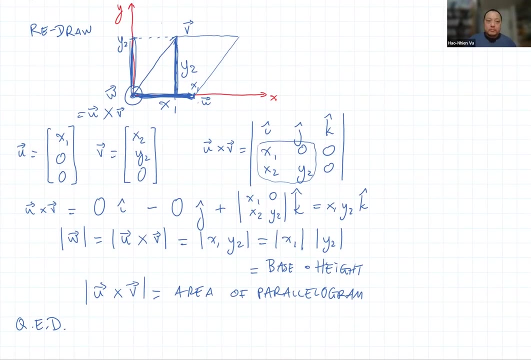 Base times height, And so the whole thing is Well, that was fun. But before I close, let me say this: